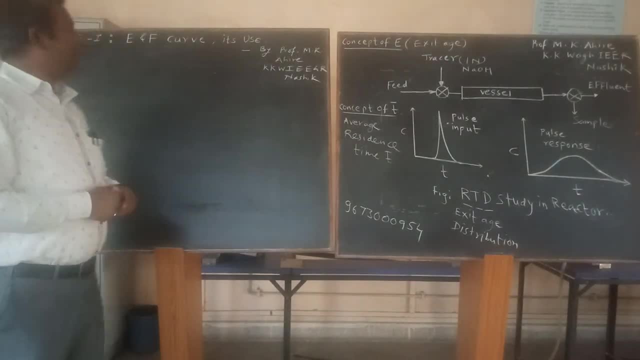 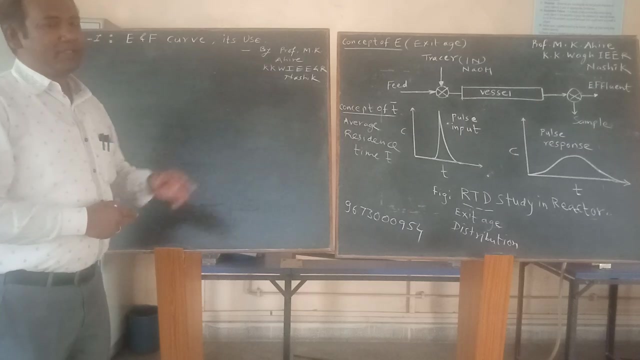 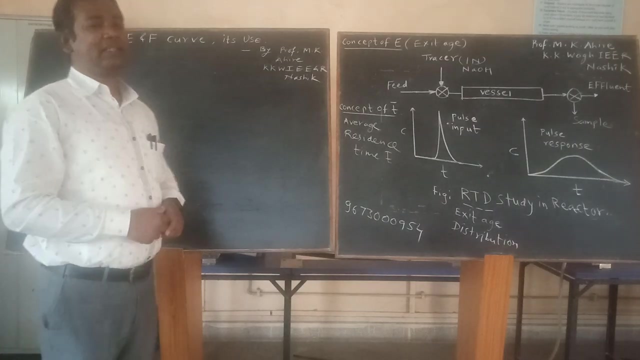 Hello friends, let us discuss what is E and F curve and how it is useful in determining the residence time and in determining the flow pattern or mixing pattern in the reactor, in continuous reactor. In previous video we have discussed the experiment and we have discussed how to find the different quantities and also we have discussed how to find E. also, From E we can determine T bar. also we can determine sigma, sigma, square, these values also. 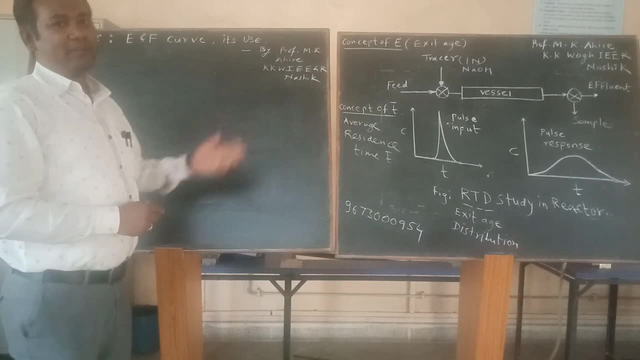 So, if you want, you can see that video first and then you can have this video for your enriching your knowledge. So let us continue. Let us continue with E and F curve. Now, as you know, E is your C i value C i is that instantaneous concentration divided by total concentration. 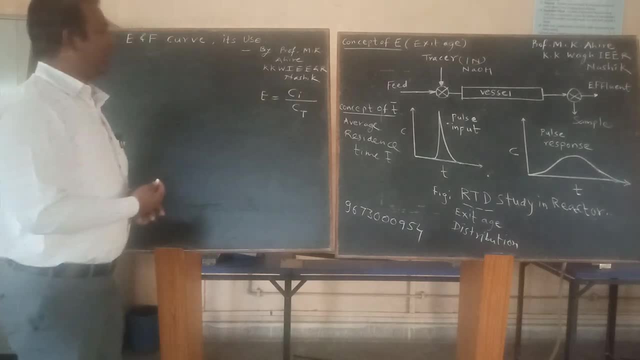 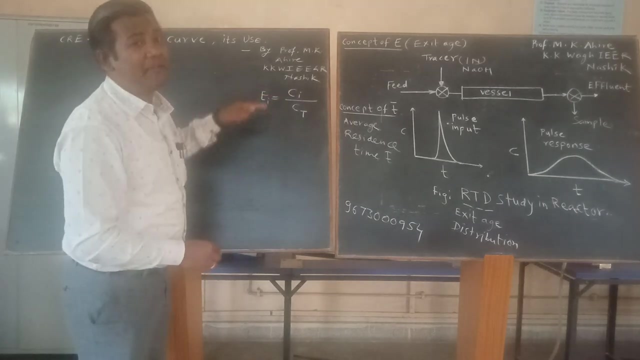 That ratio is called as exit edge and this exit edge value is totally depend on that concentration, that instantaneous concentration. So there may be, If we, If we have 40 readings, we will have 40 different values of E- i. So it means you can plot E i versus T. 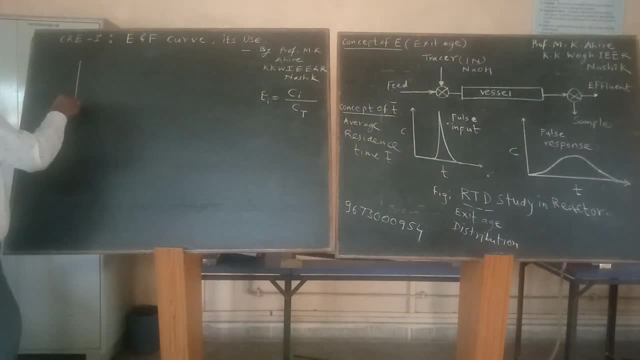 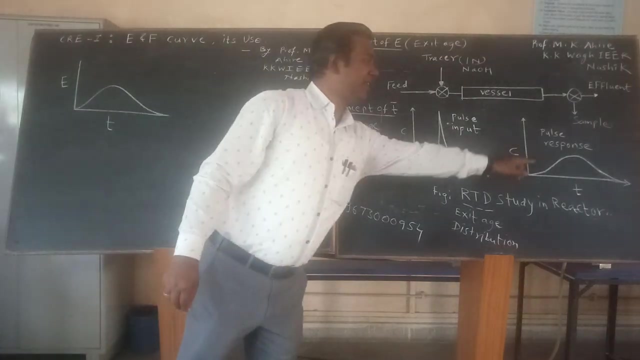 So that is the E curve. So this is E versus T graph. So this graph is just like your C- T curve, C versus T curve we have already known. So this is the C versus T curve. Exactly like that this E versus T curve is. 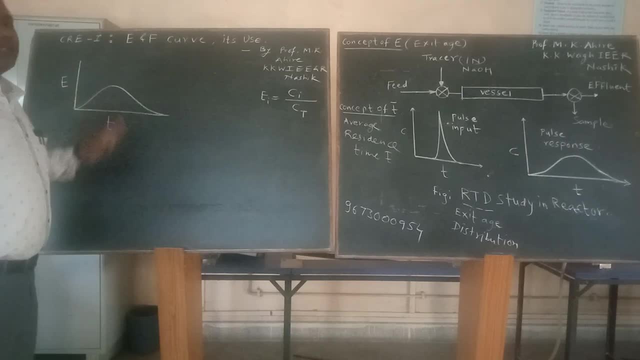 So actually, what is the significance of this curve? First, try to understand the area here. E, T 0 to T. EDT is always 1.. Means, if you calculate this area by any means, by numerical integration technique or by graphical way, what you will get. 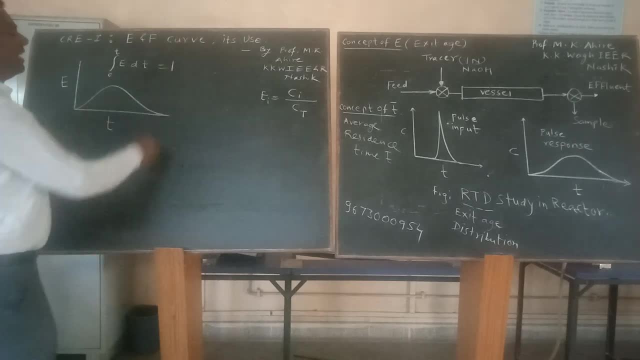 The total area is 1.. 1 indicate 100% pressure. So this indicate that 100% pressure is now out of the reactor. So this is the value of this E curve: That area under E curve is always 1.. 1 indicate 100%. 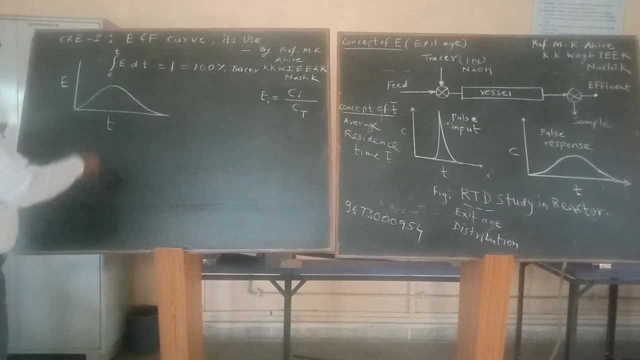 Now how it is useful. Let us consider: You have to calculate How much percentage of material has spent A certain time. Let us say this is 0 to 50 minute time interval, And if you are interested in finding out That, how much material has spent 15 minute as a time, 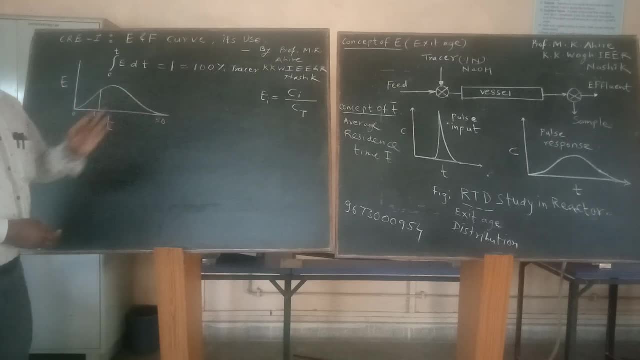 Up to 15 minute as a time inside the reactor. So what you have to do, You have to just draw a vertical line from 15 minute And you have to just calculate this area. So this area is what It is: 0 to 15.. 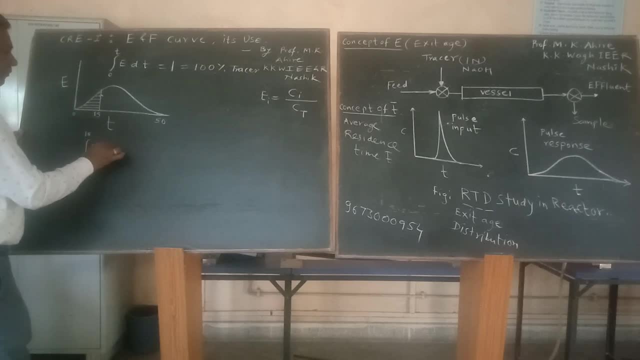 EDT. And what is the value X value you will get? It will be a numerical value. It will be a fraction less than 1.. Let us say it is 0.3.. So what it means? It means 30%. 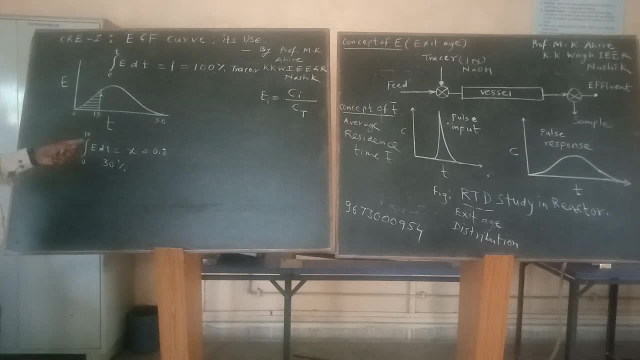 30% material has spent time Maximum 15 minute inside the reactor. 0 to 15 minute inside the reactor. That is the minimum If you want to find How much material has spent time between 15 minute to, let us say, 14 minute. 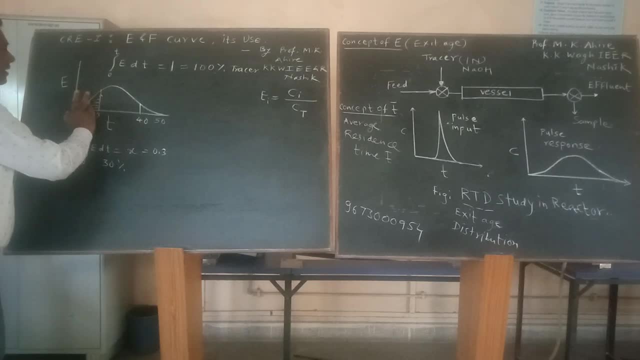 What you will do Then. you will consider this area, This area, So this area. you will consider: Ok, So area between 15 minute to 40 minute. You will consider that, Let us say that area is 15 to integration, 15 to 14.. 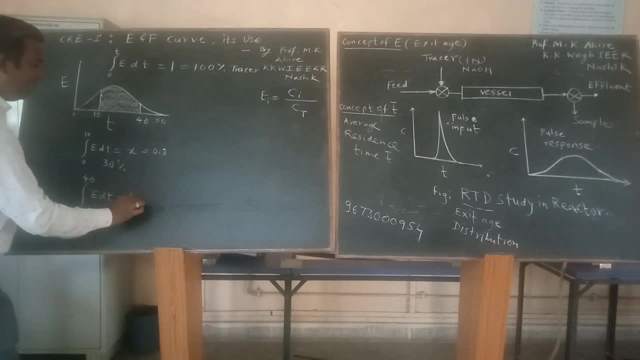 EDT is 0.6.. Let us say it is 0.6.. So what it means? It means 60% material has spent time between 15 minute to 40 minute. What is the clear cut meaning of this? Ok, 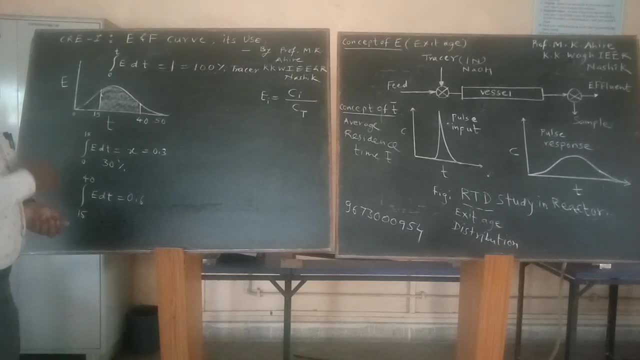 So this way you can determine how much fraction of material has spent how much time, And this is called as a F. F is We can define F. Let us say 0 to T1.. Means EDT. So what is the meaning of this? 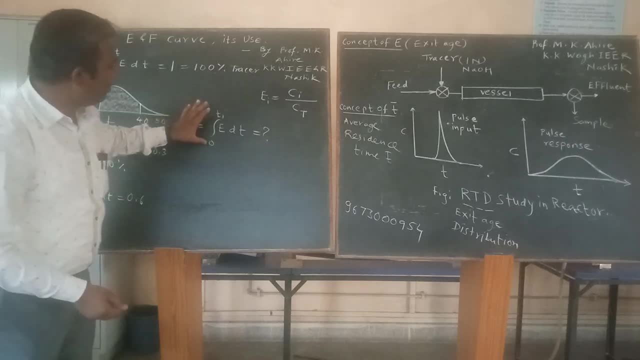 It means fraction of material Which has spent time between 0 to T1 minute Is indicated by this F. We can say it is F1.. Ok, Let us say: if you want to calculate further values of F, You will just add more time. 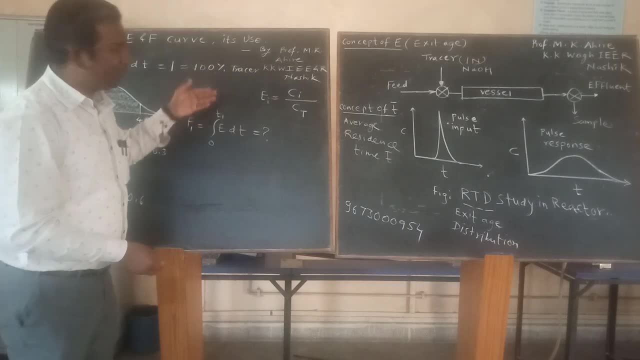 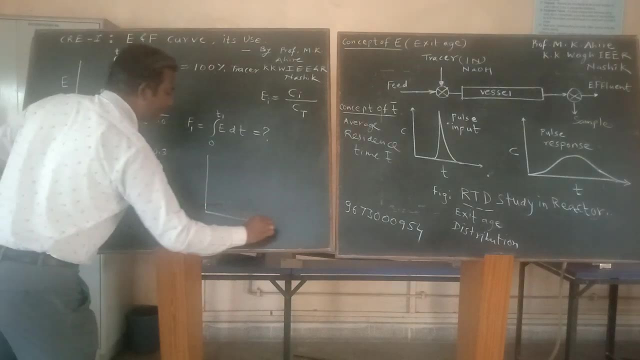 So 0 to T2,, 0 to T3,, 0 to T4.. In this way you will get different values of F And in this way you can get a curve, F curve, And that is just like this. So this is the F curve. 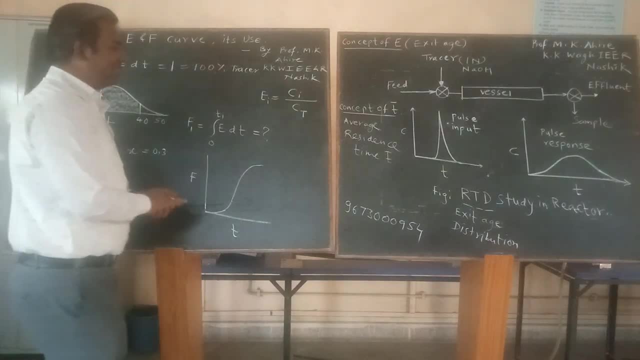 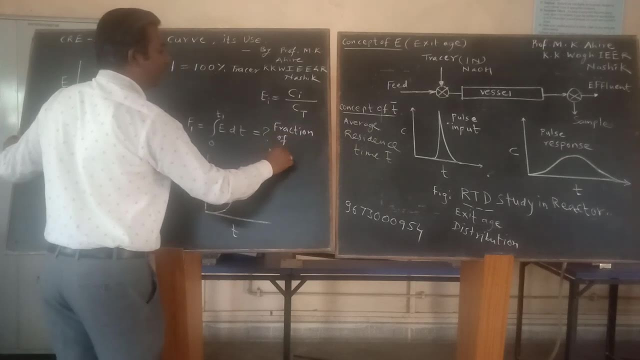 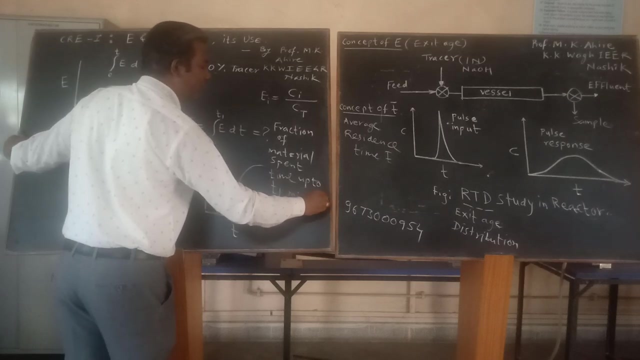 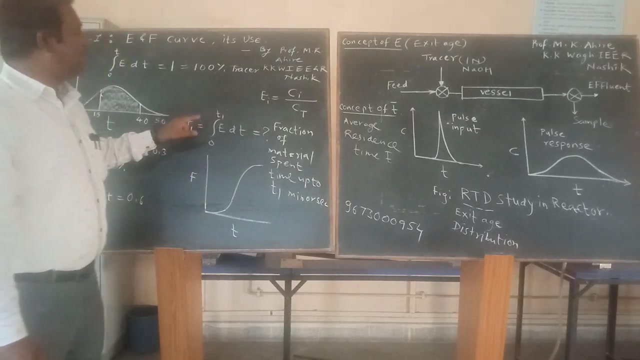 Getting from E curve. So F is what It is: the fraction of material spent time up to T1.. T1: minute or second, Or whatever that time is. So this is what The value of F, Which is we are getting from E curve. 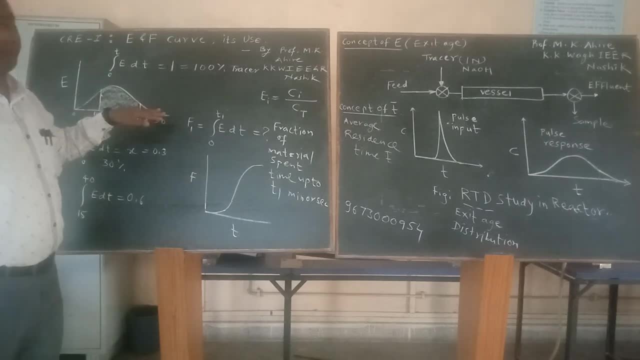 So F value you are getting is from E curve And maximum value of F is 1. Because integration EDT is maximum 1.. Ok, And 1 EDT is 100% interest rate, Ok. So in this way you can find different values of F at different time interval. 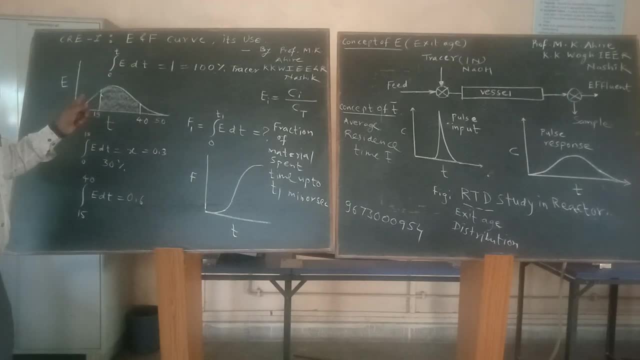 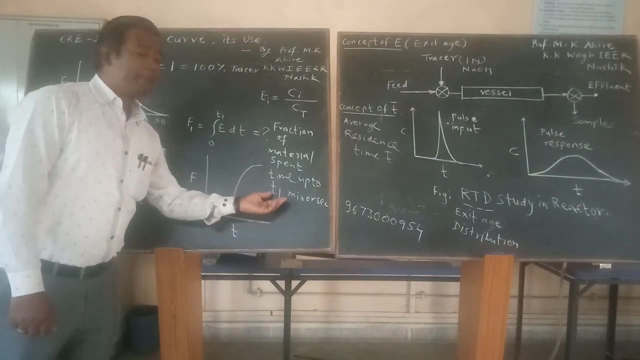 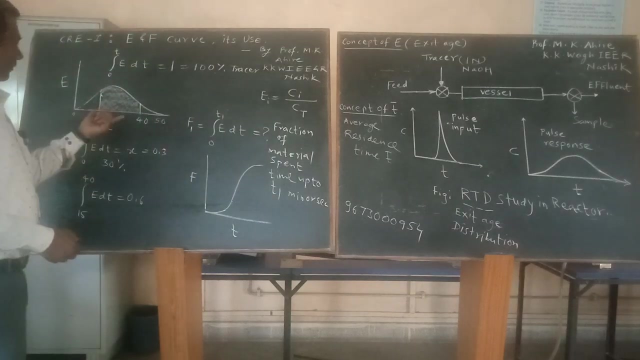 And you will get this curve from this. So F curve is totally depend on E curve And what knowledge you can get is You can get that how much fraction of material has spent, How much time interval. Ok, Let us first revise.